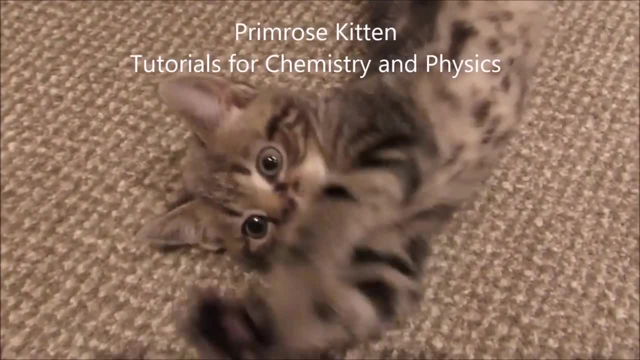 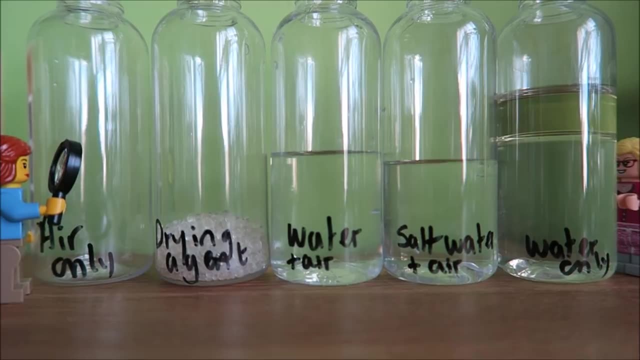 Hey guys, today we're going to be looking at an experiment about rusting. So in this experiment where we're looking at rusting, I'm going to set up five different conditions. I'm going to set up air only. I'm going to set up something that has a drying agent in. 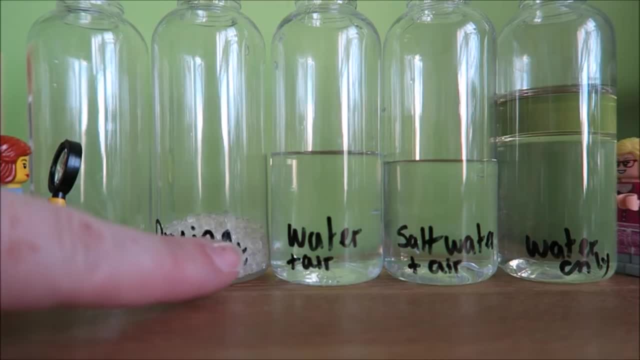 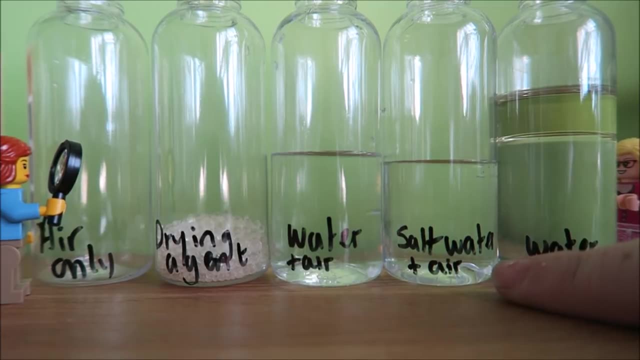 which is going to remove any moisture from the air. This is just water in here, so this will be water and air Here. I have salt water and air, so I've just taken some water and added some normal salt to it, And this is water only. This is boiled cooled water with a layer. 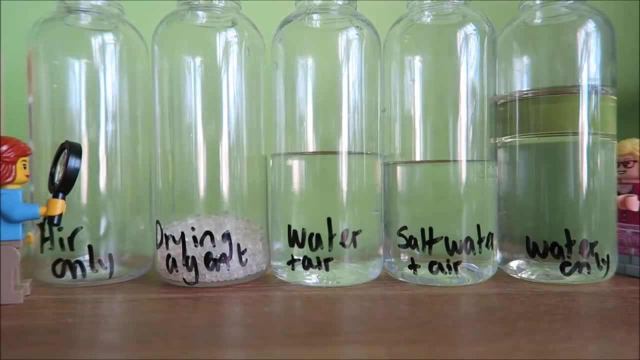 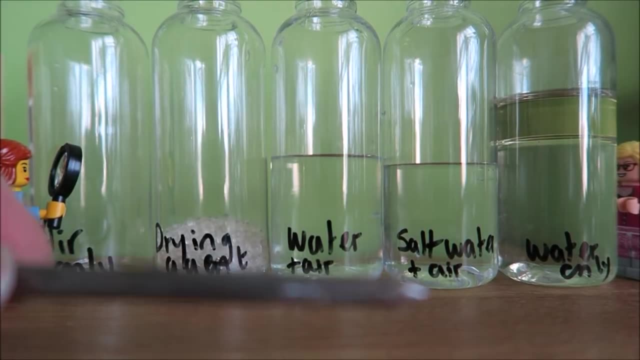 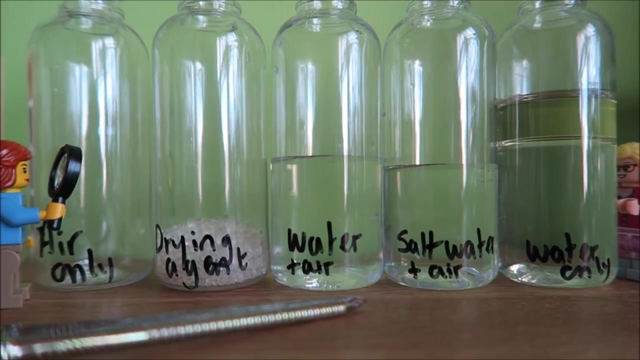 of oil on top to stop any air getting in. And to each of these I'm going to add two different nails. I am going to add a normal iron nail and I'm going to add a galvanized iron nail. Now, the galvanized iron nail has a layer over the top of it. This is of a different metal. 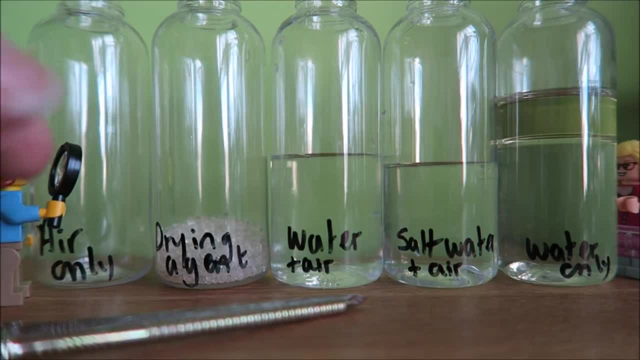 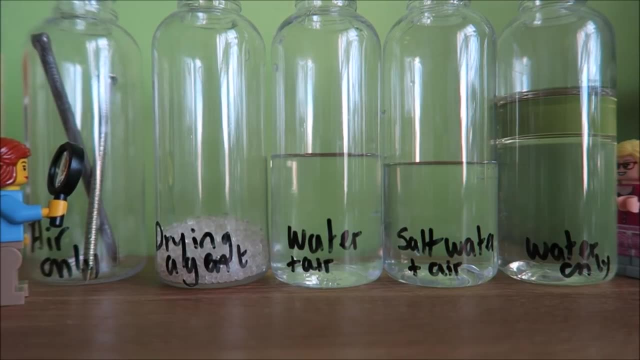 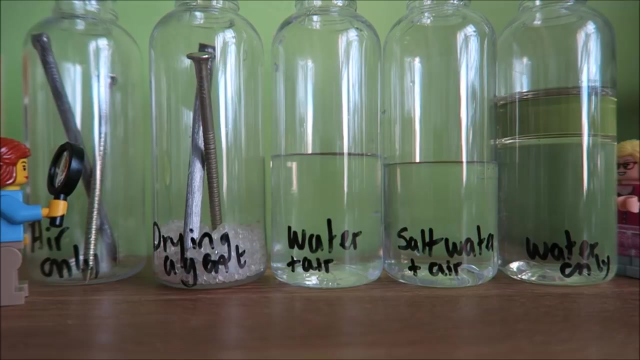 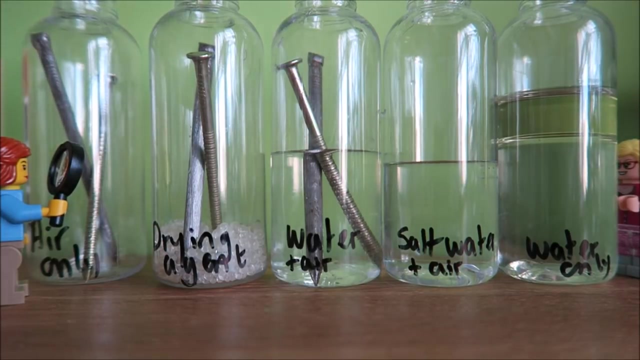 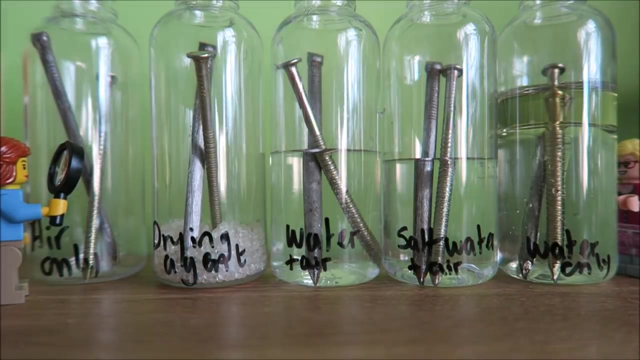 and the idea of this different metal is that it's going to stop it rusting. So two nails going into each condition And I'm going to leave these here for a few months. I'll check back in periodically with them to see what is happening and then I'll show you the results right at the end. 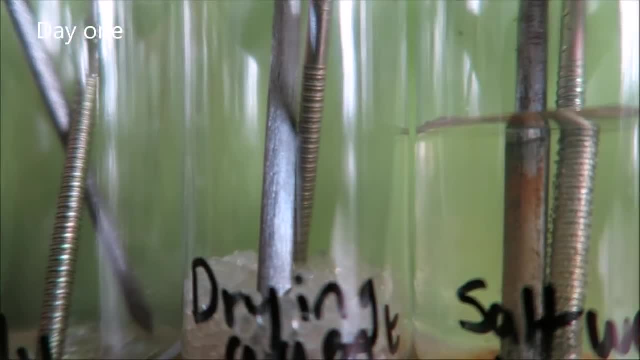 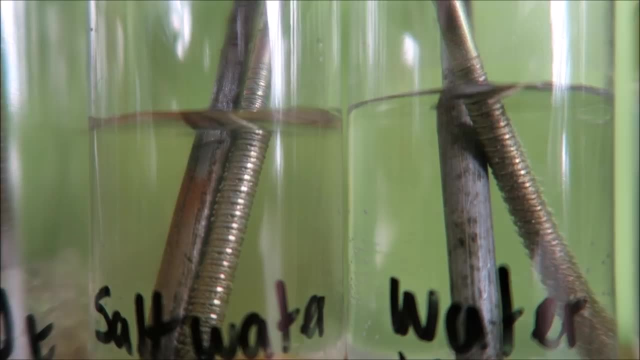 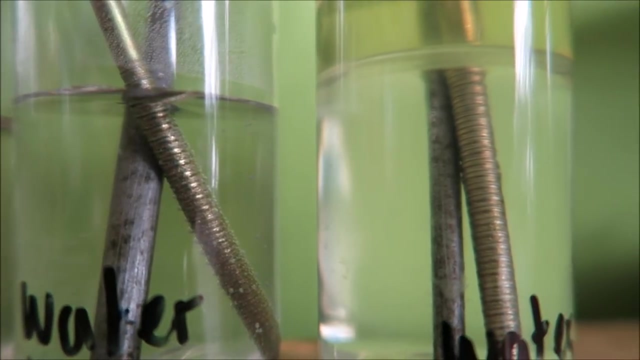 So day one and we can see that the air and the drying agent look pretty clean. But the one in salt water and the one in water have already started to go quite rusty. This is quite a surprise. I didn't think they would go rusty this quickly. And then the one over here in 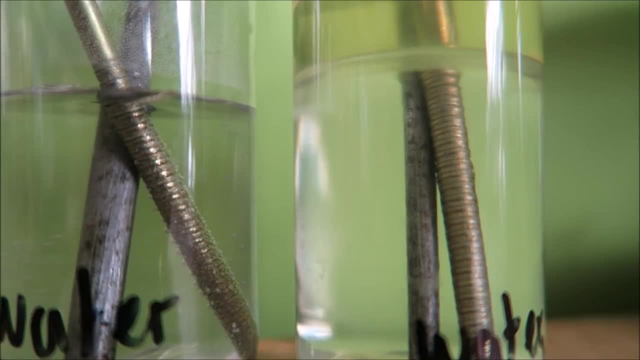 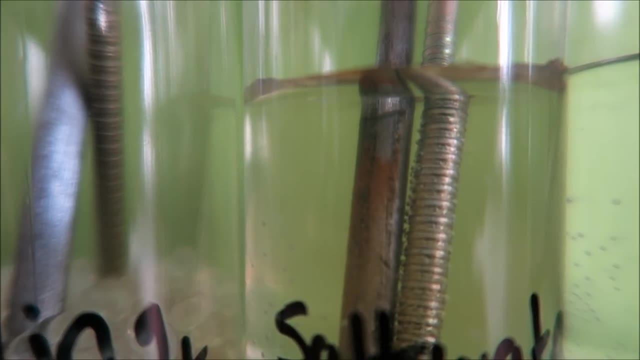 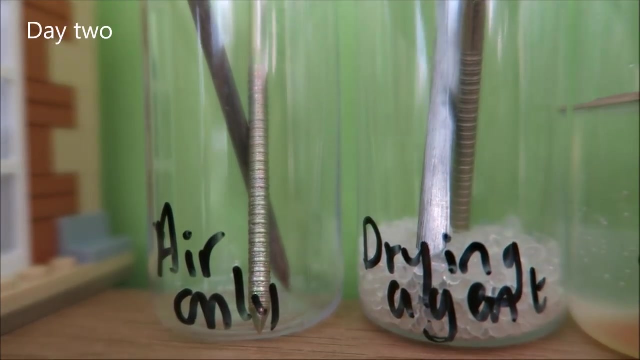 oil and water. you can see that that smells, maybe, but maybe not. So you can see that the one here in salt water is really starting to get quite rusty, whereas the galvanised nail in there now isn't Day two of our experiment And you can see that the nail in air is starting to go a little. 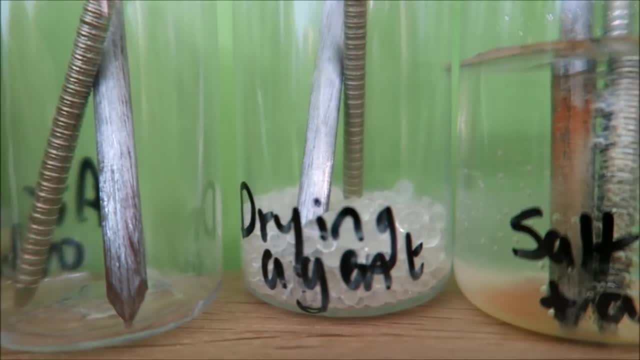 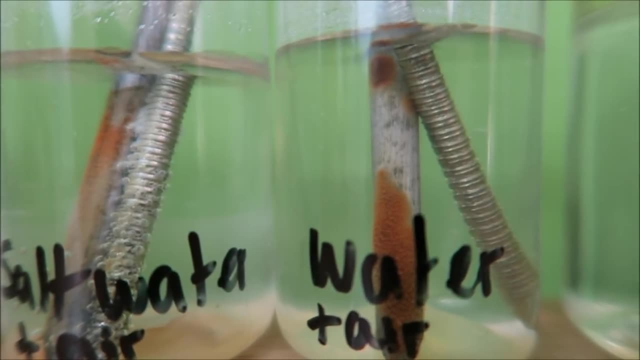 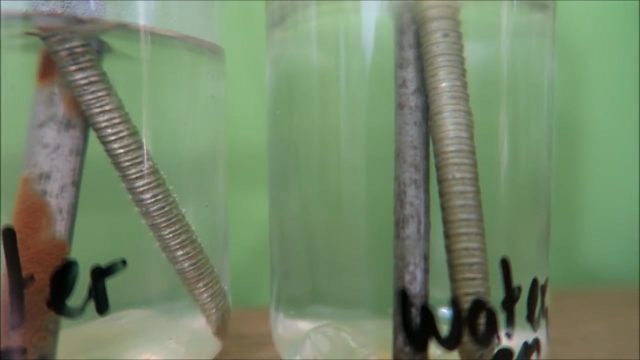 bit rusty a little bit down the bottom there And the air and the drying agent looks clean and shiny. it looks well pretty manky. now and again in water it's starting to go rusty. the one over here in water only looks pretty clean. maybe a few little bits in there, but nothing compared to these two. 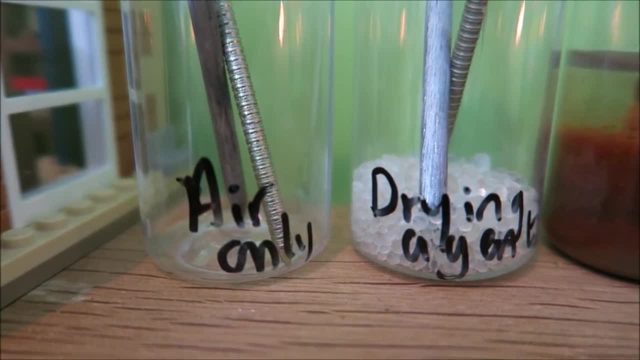 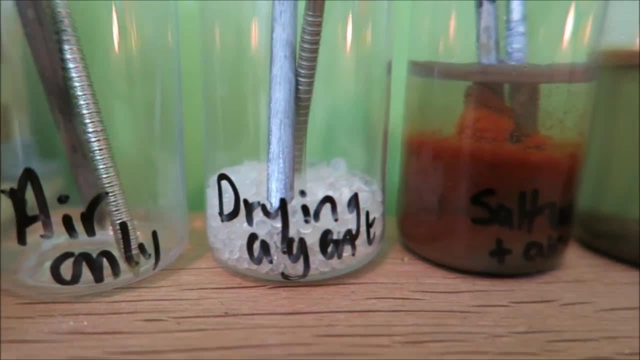 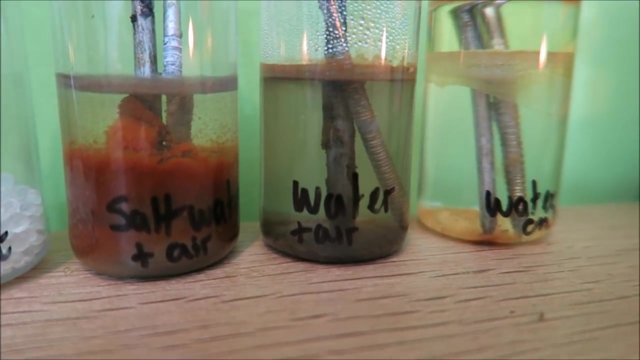 over here. here are my nails. it's been a few months now. we can see the air one is looking a little bit tarnished, the drying agent looking very shiny, the salt water and air that is just full of rust. the water nails look a little bit manky and then the water only is looking okay. over there i'm 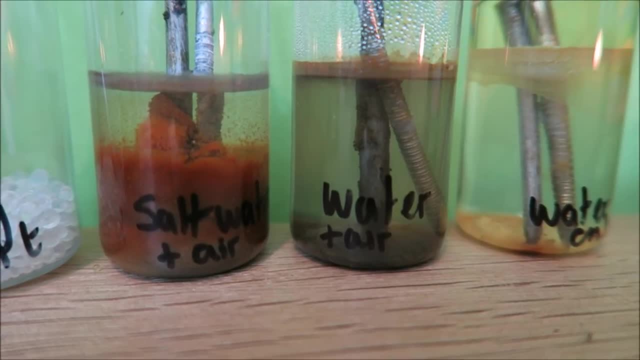 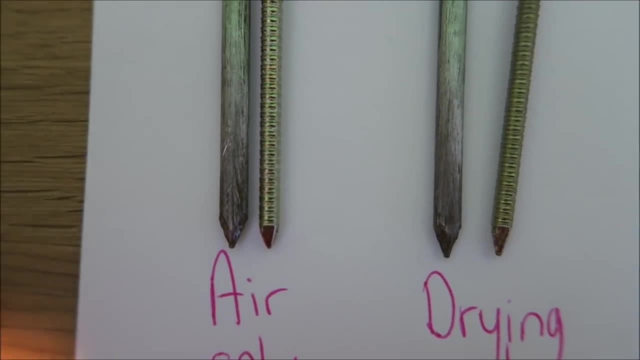 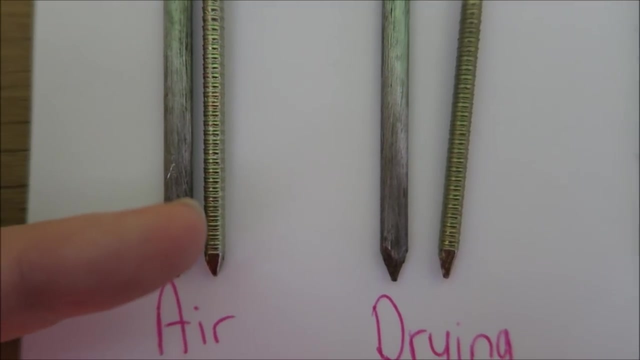 going to get those out and show them to you all properly. so here are the results you can see with our air. only the iron nail is looking pretty good. i was hoping this one would go actually quite rusty, but i guess my um set isn't very um humid. and then the galvanized nail next to it looks 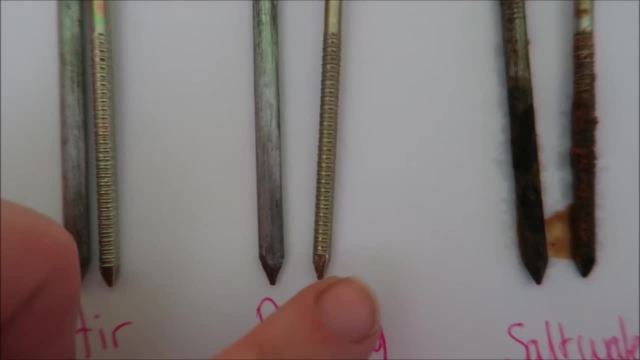 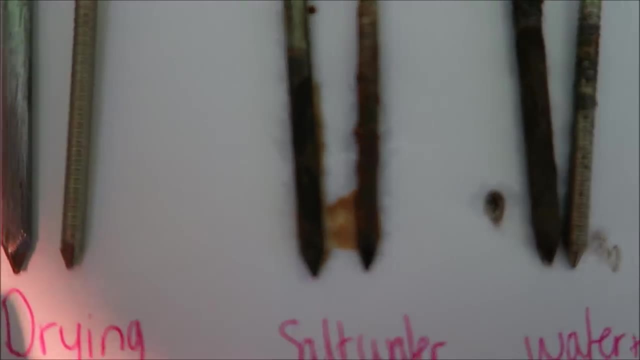 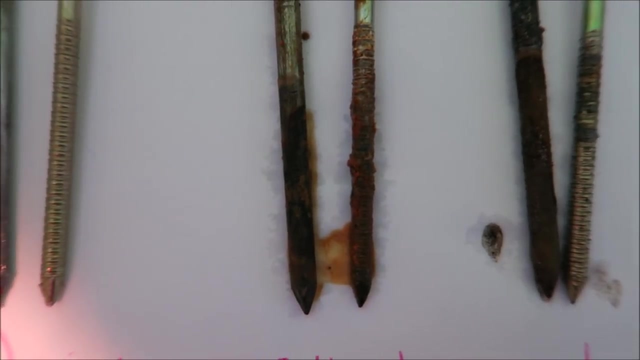 perfect the drying agent. again, it looks pretty good. and then the galvanized nail next to it. basically no rust on there at all. now, here we have the salt water and air. you can see this now looks pretty bad. both of these nails look pretty bad. um, there is rust all over them. you can see. 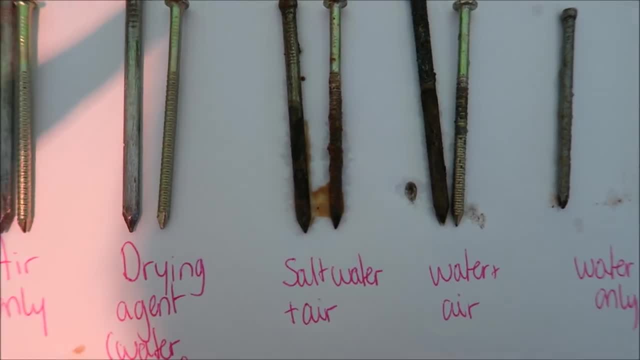 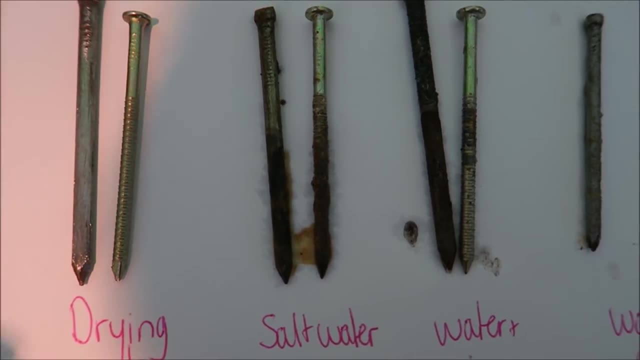 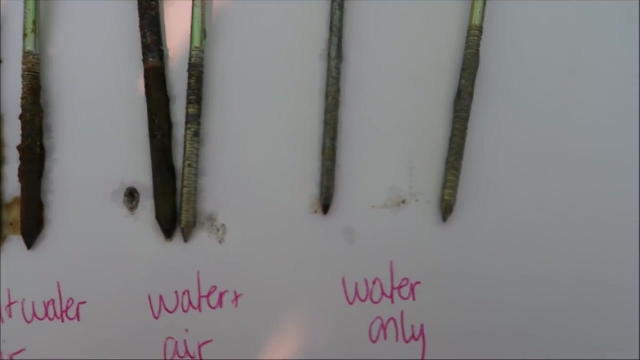 that the paper that i've tried to get out. um, it is covered in rust and if you remember back to what the jar looked like, what the bottle looked like, it was full of rusty bits. here we have water only and that's full of rust. um, now, with the water that i'd boiled to remove the air and then put the oil on, 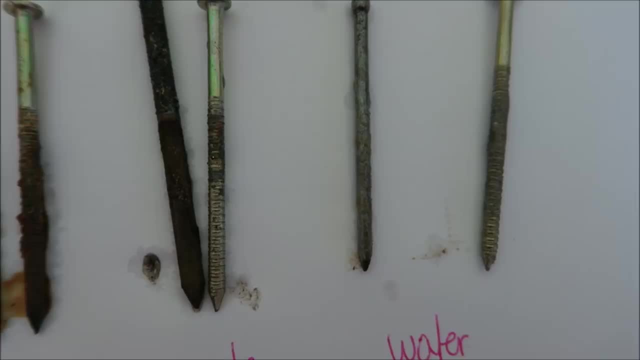 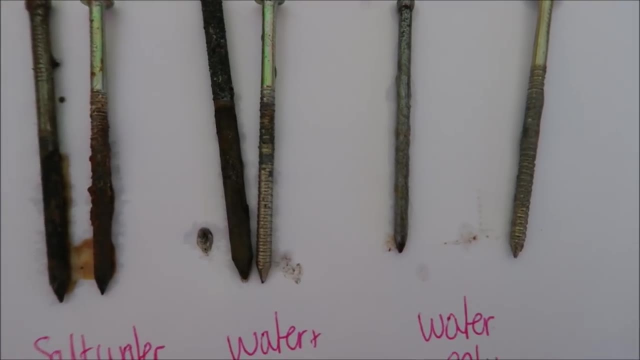 top so that, um, no air could re-dissolve in it. you can see this doesn't look too bad. it's a little bit manky but i think that's probably because she's been seeing in water and oil for a couple of months, but it's not really rusted. if we just go back over here we can look at the galvanized nail. 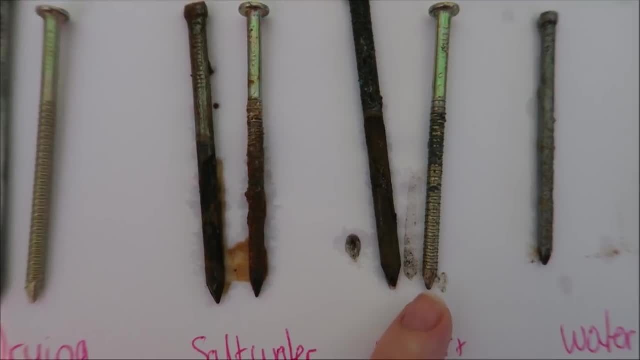 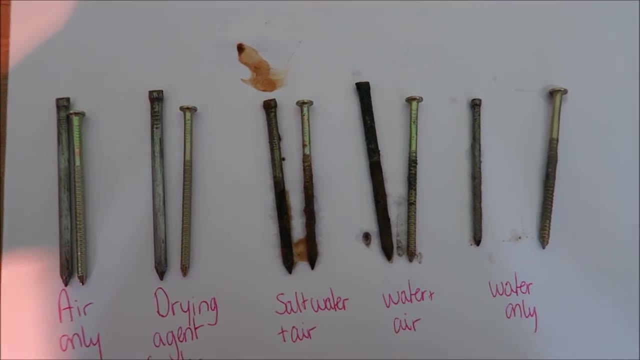 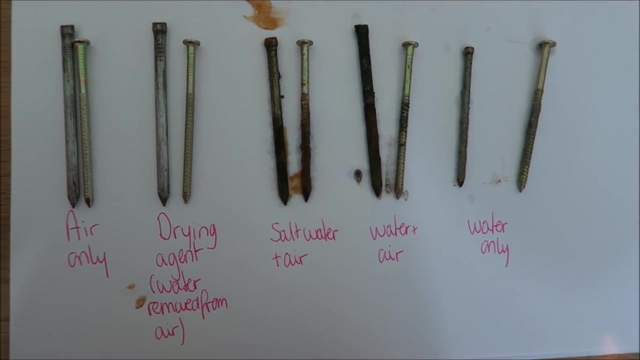 we can see, this actually looks pretty good. it's a little bit manky, but it's not as bad as this nail here, which is really, really horrible and rusted. so from our results, we can say that the two things we need for rusting to occur are water and air, so the equation for this reaction is iron plus water.